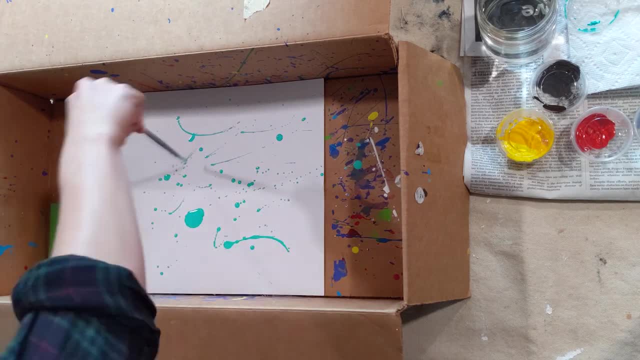 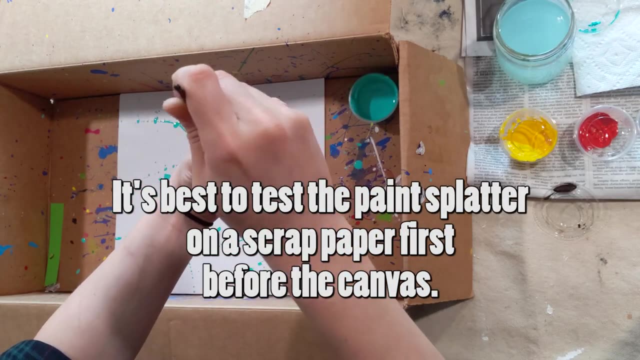 You don't want it to be too watery, So you just add a little bit of water, test it and then, if it's the right consistency, you're good to go. So I tested it out with this one, but then I went and mixed each color after that to prepare. 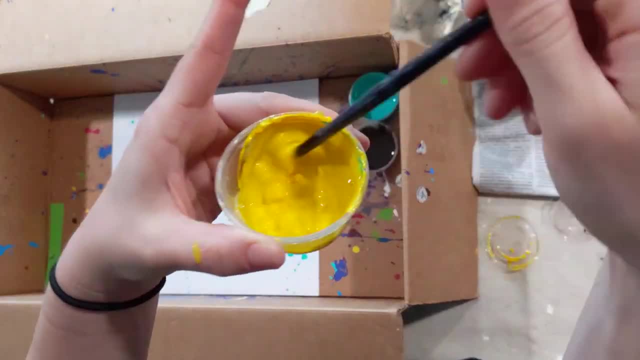 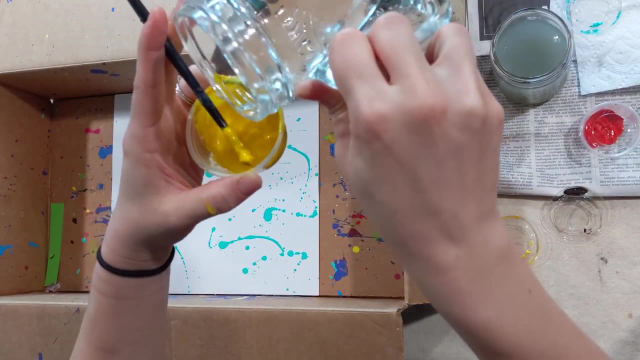 You want to mix it until all the clumps are totally mixed in. The paint should should be one consistency, so you don't want it to be lumpy. you want to mix, mix, mix, mix, mix until it's all one consistency and a little bit drippy try. 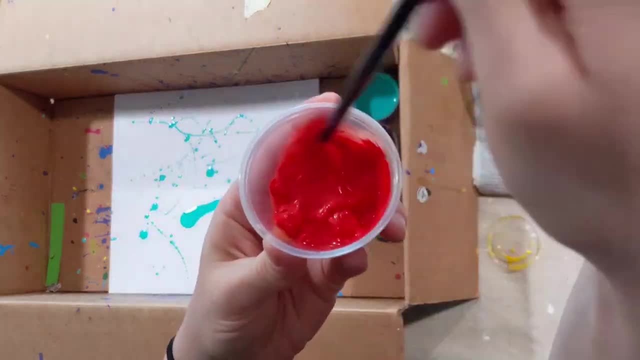 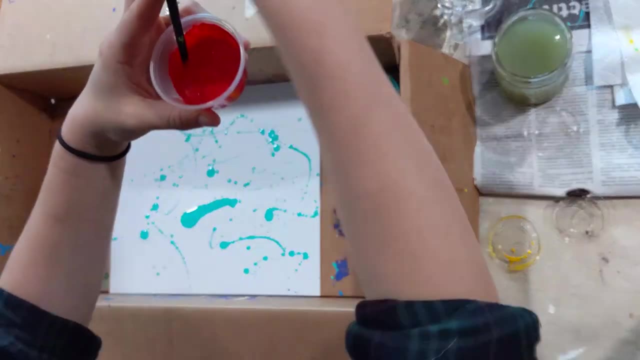 adding a little bit of water. mix it, look at it, see if it drips when you tap it. if it doesn't drip when you tap it on the lid, add a little bit more water, mix, mix, mix, mix, mix and then try it again, see if, when you tap it on the lid, on the ledge, 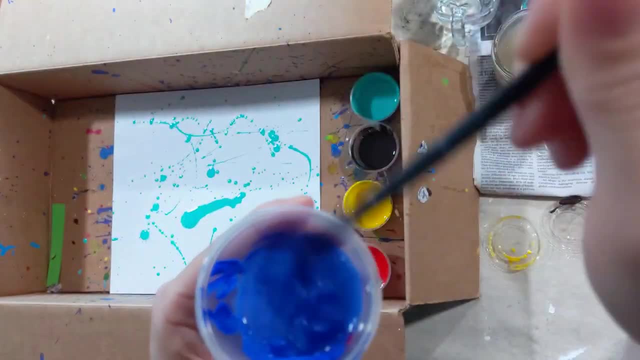 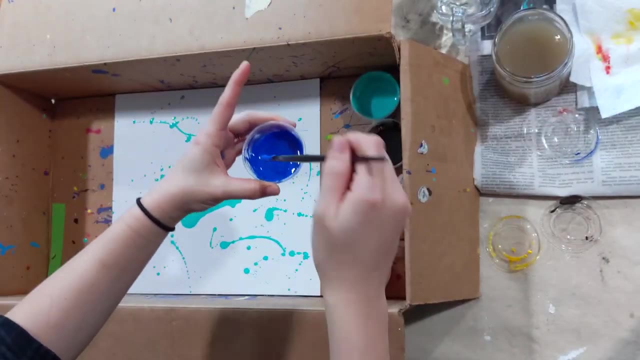 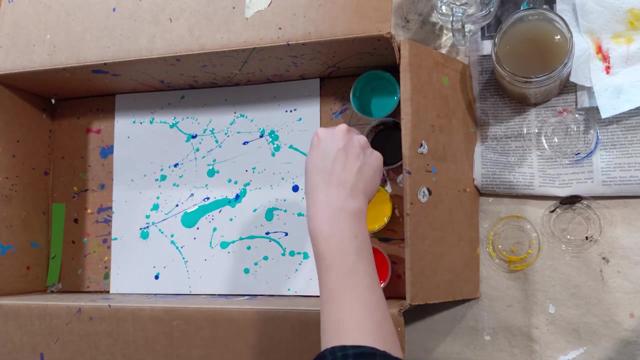 if it drips. once all your paints are ready to go, make sure you pick colors that you like, that you're gonna want to play with. you don't have to use all your colors. I chose five colors that's actually brown, not black, and then I tried different types of drip techniques, like Jackson Pollock, who we are kind of. 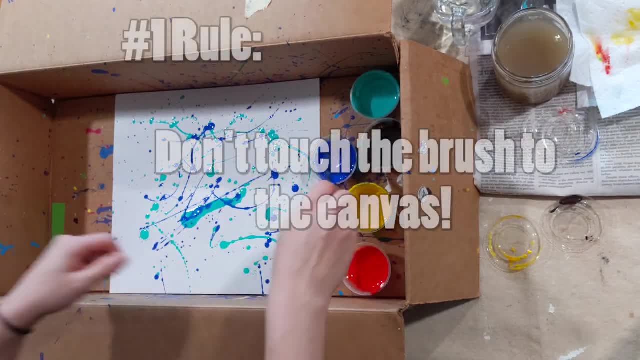 basing this off of the number one rule is: don't touch your brush to the canvas. it's all about action. you can even put a song on. you can listen to a song or you can listen to a song. you can listen to a song or you can. 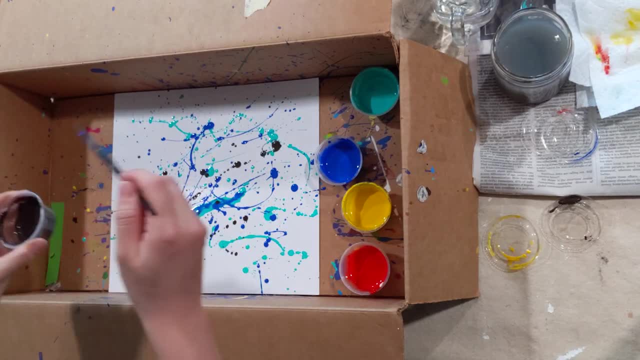 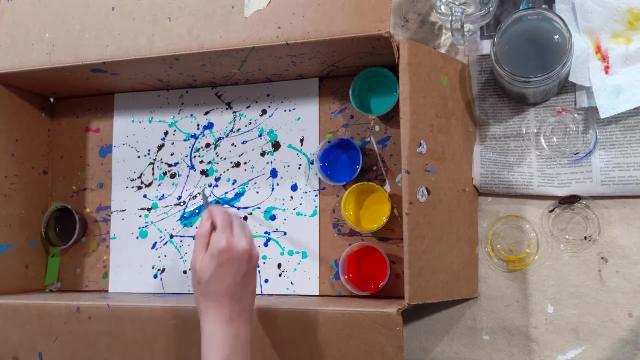 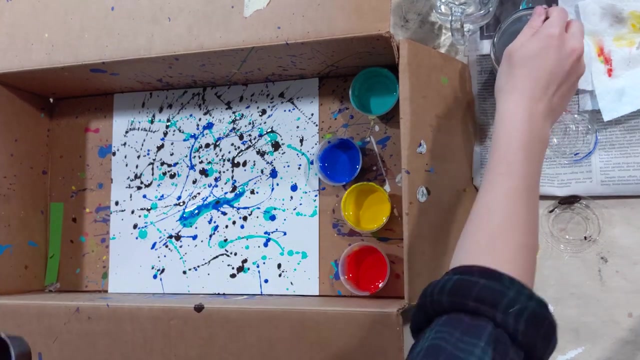 listen to something that gets you into a movement of some sort. there's different ways to do this, but we we want you guys to just really feel the painting process, just really have fun moving and getting that movement onto the paper without touching the paper. some flicking methods are really cool. sometimes I tapped it on. 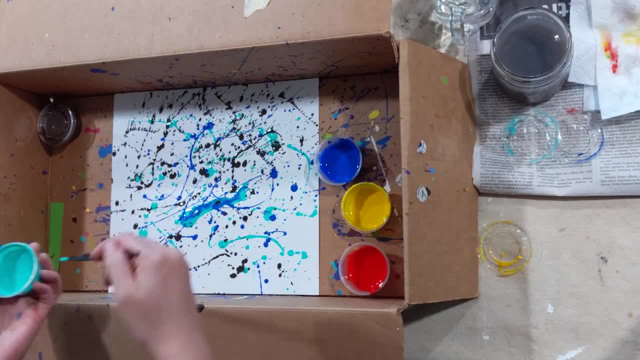 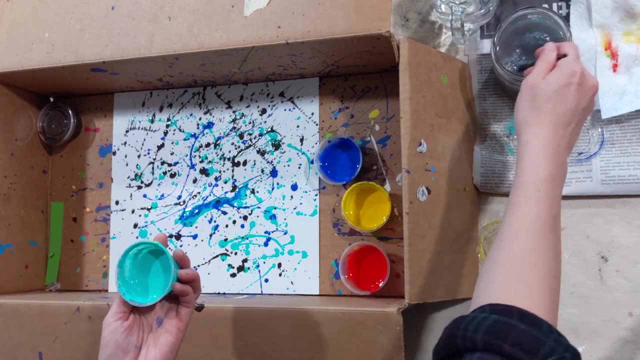 the edge of the box to try to get some drips. sometimes I even just poured a little bit of paint on there. it's a great trick: just a little bit of paint and we're really going to go through the process of getting more paint and go with the flow. just flick it, act like a 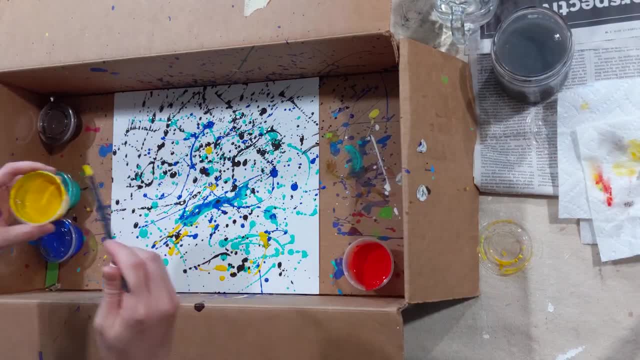 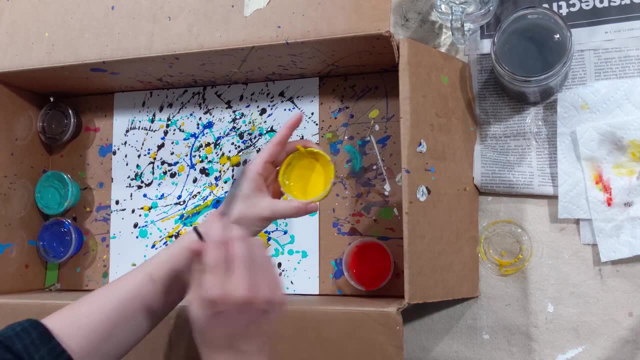 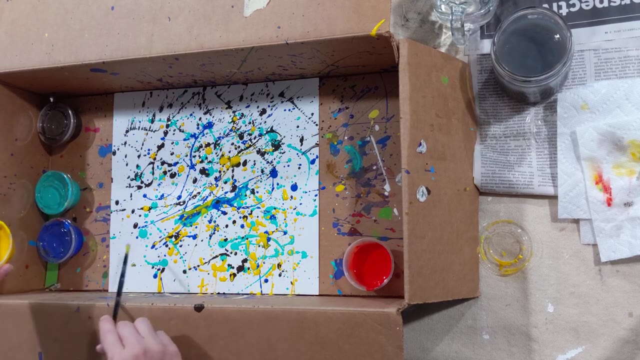 music conductor and swing left and right. just make sure that you don't get paint all over your house. the paint will go everywhere, so try to stay inside the box. keep your mess to a minimum for your family's sake, so that we don't have a lot of mess to clean up. I saved red for last because it really pops. it's my.